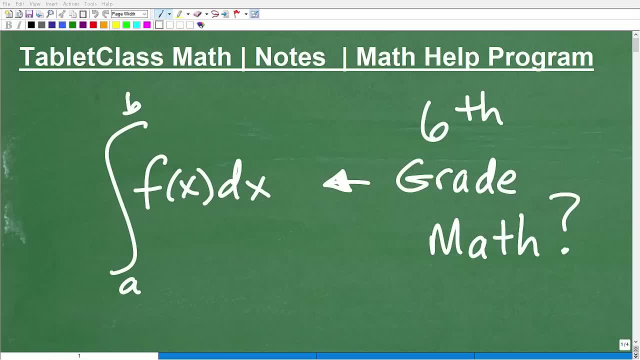 Okay, how would I explain calculus to a sixth grader? So here we have a little question here: Is this sixth grade math, And what we're looking at right here is calculus? And of course the answer is no. we don't learn calculus in sixth grade. However, the concepts we've already learned in the sixth grade is really enough to, by the time we've gotten to the sixth grade, the concepts we've learned about mathematics is enough to explain calculus to a sixth grader. 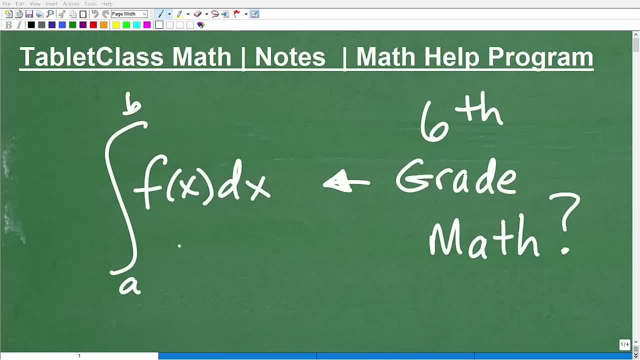 It's enough to really understand the essence of calculus and the kind of problems that can help us solve. So that's going to be the objective of this video: is really kind of demystify calculus such that anyone can like appreciate the value of it. All right, So you know most people and I can understand. you know they'll look at you know something like this, and just look so scary, Like, oh my goodness, I'll never understand that. You know, I have no idea what it does for us. Well, just stick with me through this video, You'll have a nice. 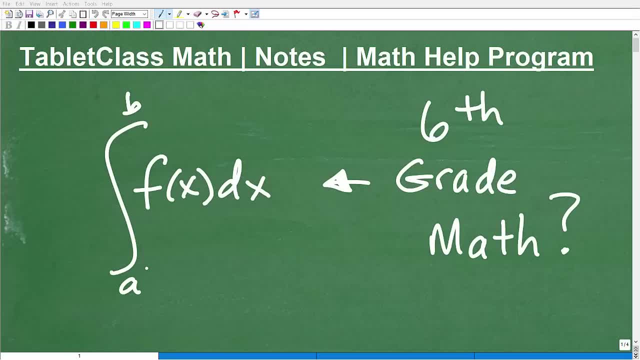 appreciation For calculus. Okay, so before we get going, let me go ahead and introduce myself. My name is john. I'm the founder of tablet class math. I'm also middle and high school math teacher, So I certainly understand what is taught at the sixth grade level And over many years of constructed full, comprehensive online math courses. So if you just need help with math or you need to take a complete math course, I'm going to leave a link to my math help program in the description of this video. Also, if you're in need of some math help, I'm going to leave a link to my math help program in the description of this video. Also, if you're in need of some math help, I'm going to leave a link to my math help program in the description of this video. Also, if you're in need of some math help, I'm going to leave a link to my math help program in the description of this video. Also, if you're in need of some math help, I'm going to leave a link to my math 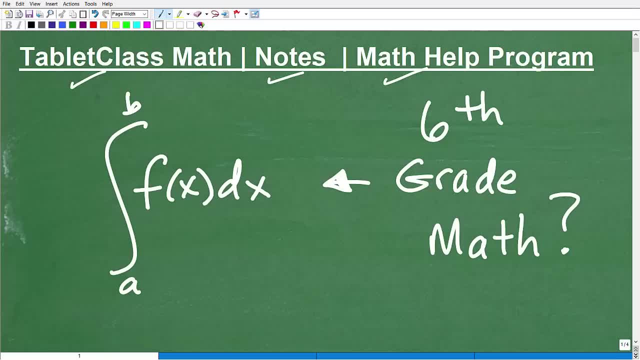 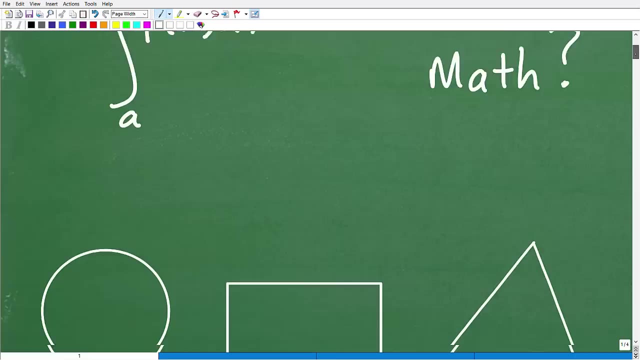 notes. you'll find links to various math notes in the description as well, or underneath this video, I believe. Okay, so, with that being said, let's go ahead and get to this topic of calculus right, and demystify it. All right. so let's start here. And I got some shapes right. I'm like I got a circle, I got a rectangle and a triangle And I said, Okay, let's find the area. 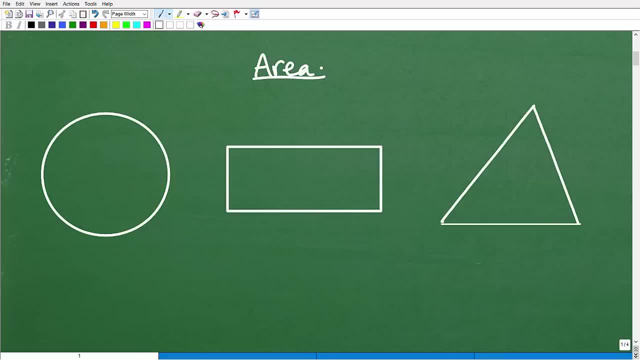 Okay, how can I find the area of these shapes? and by the sixth grade, all sixth graders and you know, and probably even earlier than that, maybe it all depends- could find the area. I certainly understand the concept of the area of a figure, right, So you might be out there, okay. well, I could find the area of a circle by using this formula: pi, r squared right, So the r is the radius, that's the distance from. 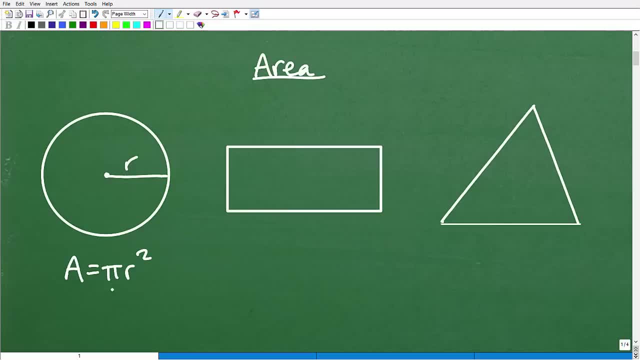 the center to the edge. But if I knew this information, I could plug it into this formula and I could find the area. Okay, like, Oh, all right, Yeah, I remember that. And here I have a rectangle. this is the length and this is the width. So how can I find the area of this guy? Well, again, I can use this formula: r equals length times width. right, Like, Oh, yep, I remember that. And here I have a triangle. you're saying, Oh, the area of a triangle is one half base times height. So this would be like the height, right here. 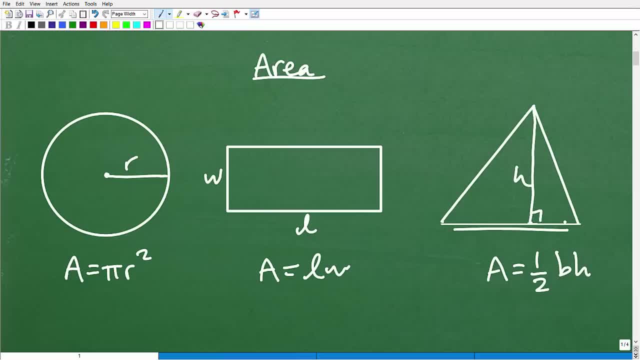 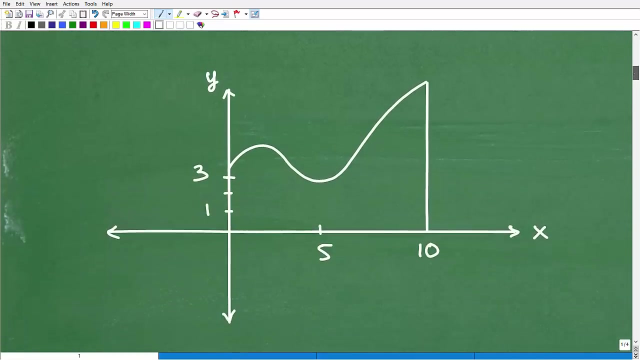 And this would be the base, So I could find the area of a circle, a rectangle or triangle. not a problem, right? So what's the secret, though? The secret is knowing the formula for those respective shapes. Okay, All right, that's all fine and dandy, But what happens when we encounter a situation like this, Like what's going on here? What if I said: find the area? 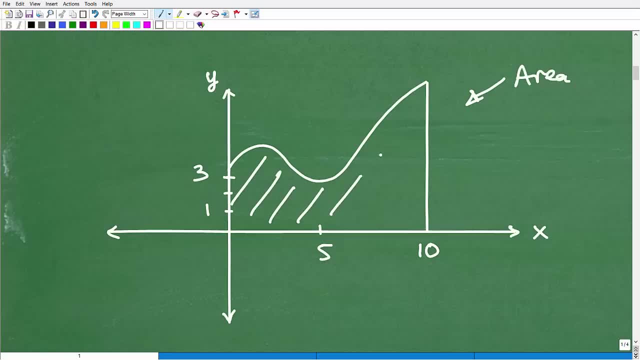 of this shape. Okay, Now, this shape is kind of bounded by this little squiggly curve and has this little border and this border and this border. So now, what do we even call this shape? It's not a, it's not a triangle, it's not a rectangle, it's not a circle. Who knows, maybe we'll call this thing a squiggly, find the area of a squiggly. And you might be saying, All right, no problem, I know how to find the area of a circle, I know how to find the area of a rectangle and a triangle and a few other things. 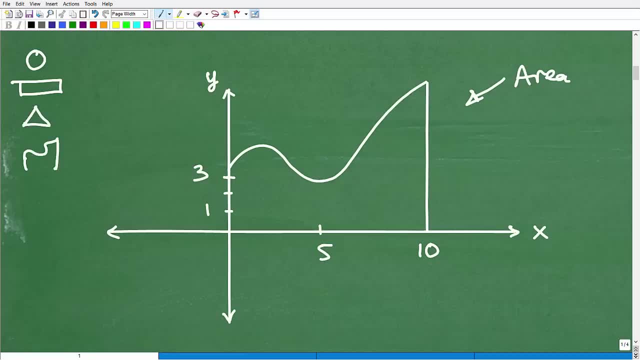 I just need to know the area of a squiggly. Okay, what's the area or the formula for the area of a squiggly? And I would come back and tell you: I'm sorry, there is no formula. There is no formula. Like we were able to use formulas. you know those nice formulas I just showed you to find the area of these basic shapes. But what about this crazy little looking figure here? Well, we're going to have to come out, come at this at a different approach. So the 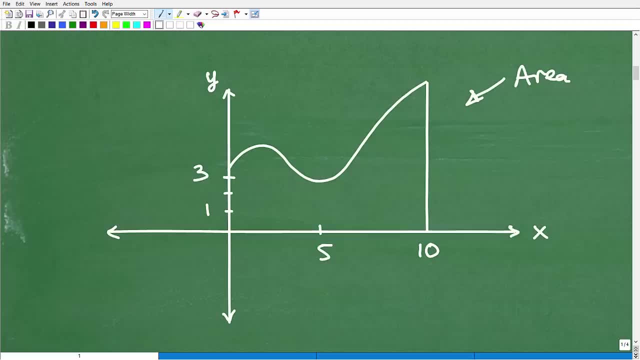 first thing that calculus does for us. it allows us to find the precise, exact area of crazy shapes. any shape that you want, you can find the area of it, And this goes for volume as well, right? So if I said find the volume of a cube, all right, so most of you might know how to do that. Or like a cylinder- we also have formulas for that. But what if I had like some crazy look, looking like like weird shape, like this? Well, we, there is no formula. 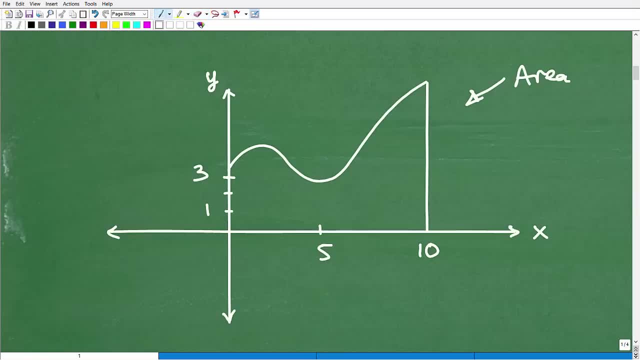 We're going to have to use other mathematics, And that would be calculus, And that's going to be our superhero here in terms of being able to find the area of things like this. Now, how does calculus work? What's the main kind of concept of no terms of being able to find the area of something like this? Well, here's how it works. So, if I said, well, just use what you know, let's just focus on the rectangle, Okay, we know how to find the area of a rectangle. 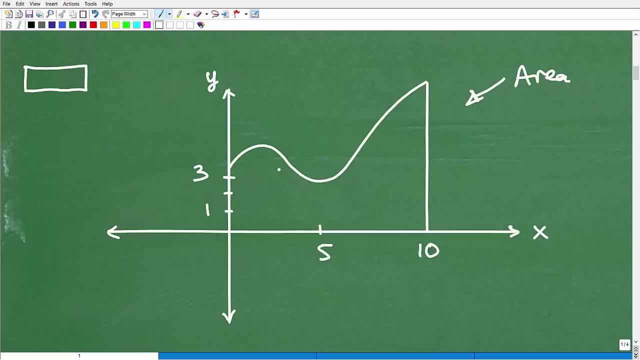 Maybe we could just find a good estimate of this little squiggly shape. So you could say, okay, let me kind of draw one rectangle here, another rectangle like this and kind of like some other rectangles, like, so you can kind of see what I'm doing. right, I can just find the area of this rectangle, this rectangle, this one, this one, this one, and add them all up And I would have a decent estimate of the area of this rectangle. 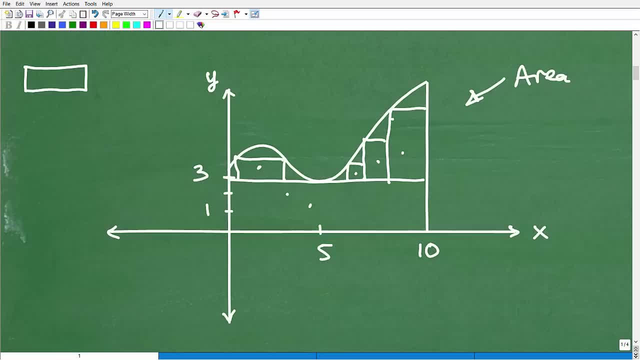 Okay, so calculus is going to be conceptually using the area of these basic shapes, precisely the rectangle. Okay, we're going to use the rectangle, but we're going to use it a little bit different way than this. But the main concept I'm trying to get you to understand is that we can get estimates of the area of anything we want by using things that we do know. okay, we do know how to find the area of these guys, So I can use little. 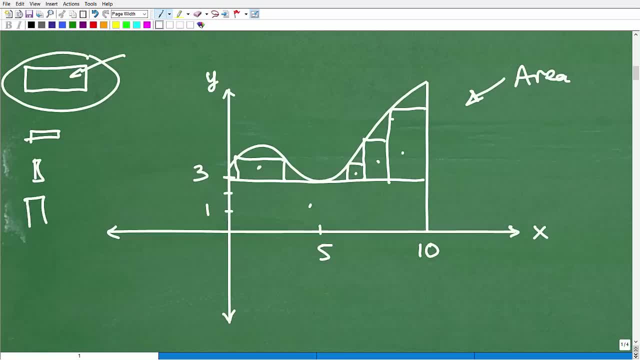 tiny rectangles, little little things, or I can use bigger ones And I could just kind of- you know kind of create that shape or estimate that shape roughly and then add up the area of all those little little rectangles. But we're going to use the rectangles more in this manner, Okay. So we're going to kind of do it like this. All right, So we're going to add up rectangles kind of vertically, Okay. 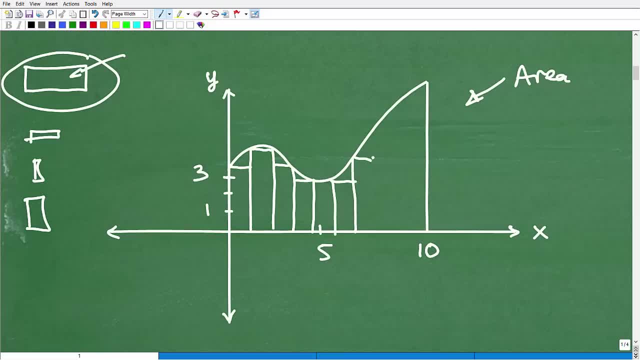 Okay, for the purposes of calculus. All right, so you can see here, these are all rectangles. Right now I have information down here. I can get these dimensions and I can get the height and I get the width. So all I would have to do that this is a better estimate than what I just showed you. Okay, I would just have to add up this rectangle, this rectangle, this rectangle, that one, all these rectangles. 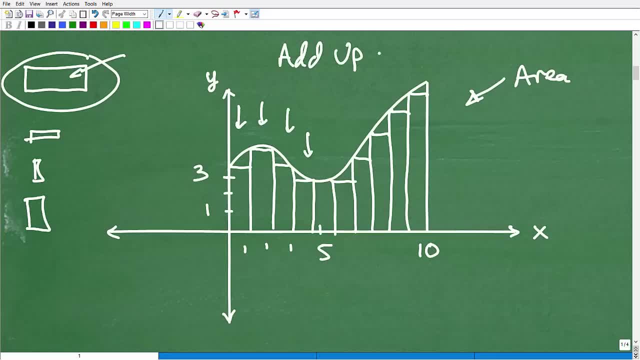 If I add up, add up the area of all the little rectangles, All right, I will get a really good estimation of my little squiggly here. Now this is going. this is where calculus is kind of heading here, right, that we're developing, or we're looking at calculus and play, Okay, like, well, so far, you know, I'm just seeing these rectangles. Well, calculus in terms of solving the 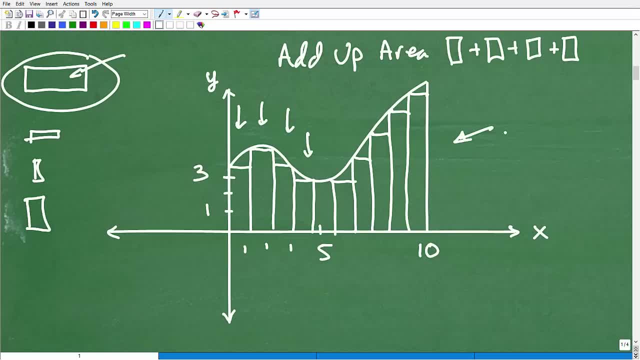 area of these crazy figures is effectively using the concept of all these little tiny rectangles. So my question to you is this: What if I said: Hey, good job, you gave me a pretty good estimation of this squiggly here, But I want a more precise answer? And you might be like: Oh, you want a better answer than that. That was a lot of work, right? That was like 12345678910, whatever, how many little rectangles So, and you had to add them all up. 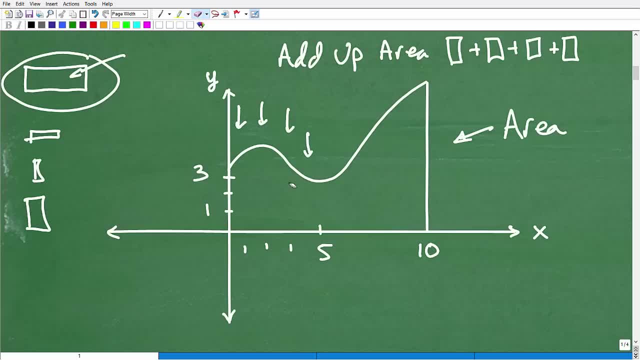 And you're like: All right, listen, you want a better estimation. Okay, fine, let's get a better estimation. How can I get a better, more precise, a super precise estimation of the squigglies? Well, you guessed it: we can use skinnier, little, tiny rectangles. Okay, Now, I'm not going to do this whole figure, But you could see here what I'm doing. So I'm using real super skinny, thin little rectangles. Okay, there's. 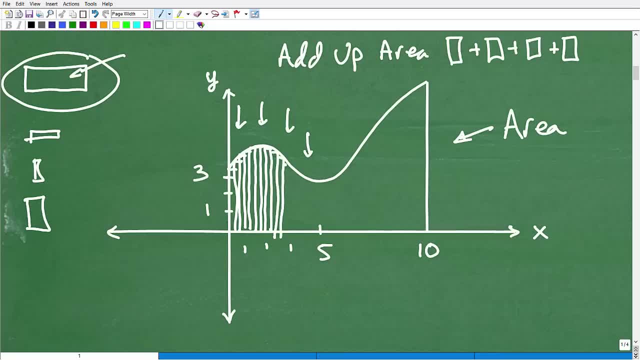 no rectangles And I still know how to find the area of a rectangle. All right, nothing's changed. But now, obviously, you can see, I'm going to have a much better estimation of the area, So I know how to find the area of a rectangle again. right, Remember, it's the length times the width, And I can get all that information here. But it's a lot more work, obviously, right, I'm going to have to add up a whole bunch of skinny little tiny rectangles. But take a look at what's going on. I mean, this is getting 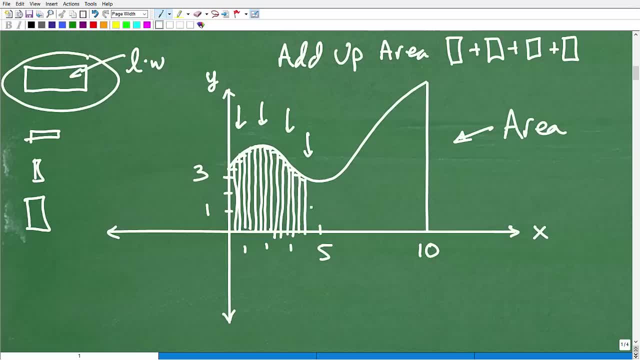 pretty nice, right? I mean like, oh yeah, this is going to be a pretty good estimate of the area of this squiggly shape, Okay. So what's the lesson learned here? Right? If I want to get a more accurate area, okay, of a particular shape, I want to use skinnier rectangles. Okay, Now, what would be like the ultimate skinniest rectangle? Well, it would be like almost infinitely. 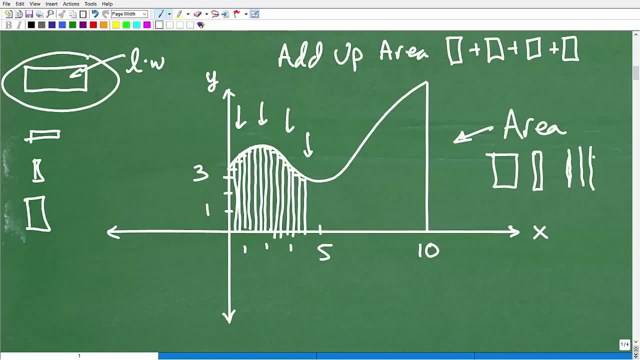 small Right, Super, super tiny, super skinny. But if I was able to just add up all these little, infinite little strips, these little tiny like rectangles underneath this, I would get the precise, the precise area of this figure. And this is, ladies and gentlemen, the main concept of. one of the biggest problems that calculus solves for us is finding the area underneath these little curves- Okay, something that's bounded like so. And so now, when we take a look at this, we'll see that the area of this figure is exactly the same as the area of this rectangle. 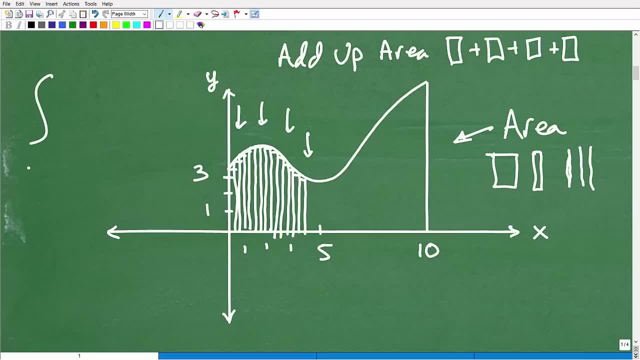 at this little calculus stuff. right, I'm gonna go ahead and say 0 to 10 and you'll see what this means here. okay, now I'm. this is actual calculus symbology. all right, you're like: all right, let's, let's understand this. what is this? 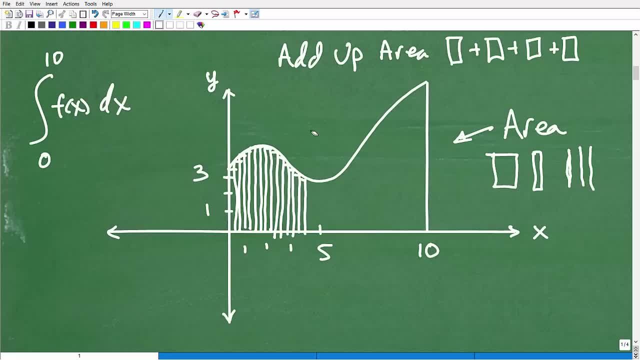 saying: well, what this is saying in calculus is the following: this little line right here, this curve, okay, this right here, can be described. it can be described in me race this with something called a function. it's just a rule. okay, it's a mathematical description of this curve. okay, it says: 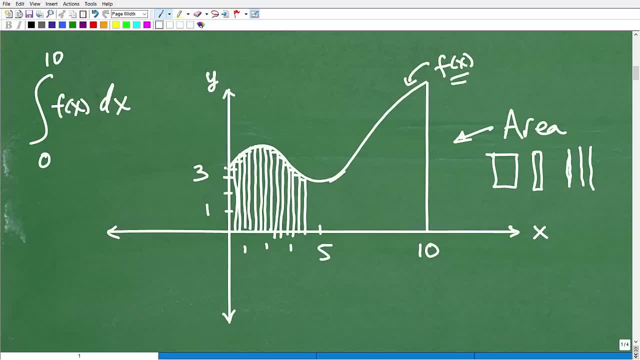 okay, if you follow this rule you'll get this curve. so in calculus, what we're trying to do, you see our little squiggly starts from 0 and ends at 10. okay, so in calculus I can say: define the area of this squiggly, start from zero, go to 10. 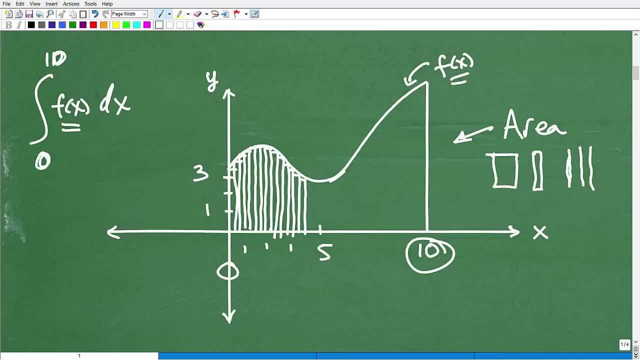 okay, okay, And we're going to be describing, or we're going to want to find the area, or we want to add up all the strips underneath this function, okay, underneath this curve, all right, Don't worry about this little notation. 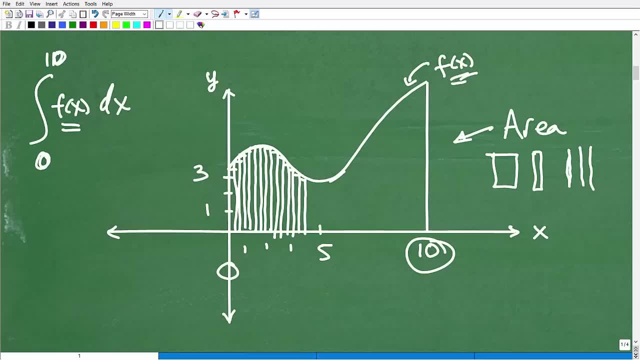 That's something that's not trivial, but we just have to write this, okay. But this little long thing right here, this is called an integral, all right, And basically it means sum okay, And effectively it means it's telling us: add up, add up from zero, start at zero, go all the way to 10, all these little, tiny, infinitely tiny rectangles underneath this function. okay. 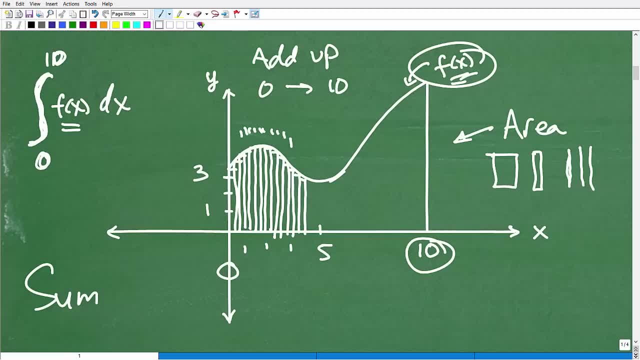 That is calculus notation. That's what that is saying. And there's another notation that kind of goes along with that. It's called a sigma notation, but I don't want to kind of get into it. But anyways, that's calculus. 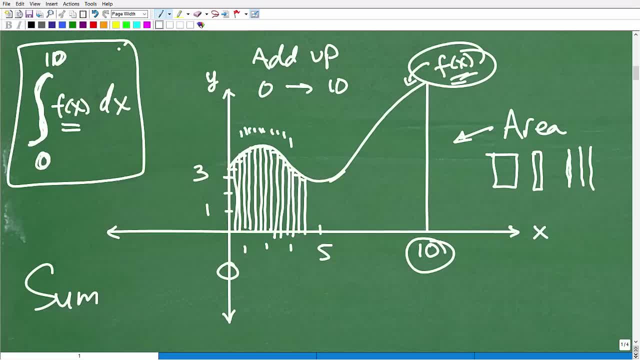 This, is it okay? Something like this is saying: we can go ahead and find the area underneath curves on a graph, right, We just need to know the function. all right, We need to know the function and we need to know where we want to start and where you want to stop. 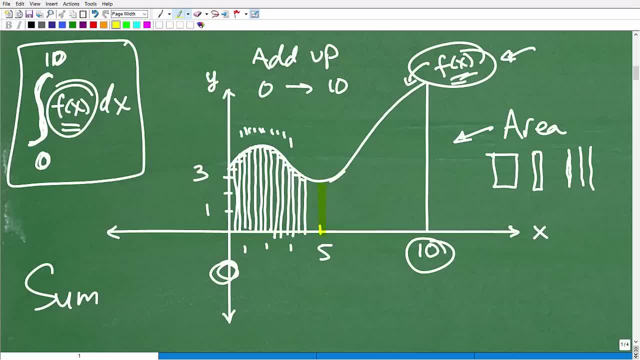 So, for example, if I wanted to find the area between like 5 and 10, okay, So this area right here I highlighted, So I would just go over here And I would write this differently, okay. 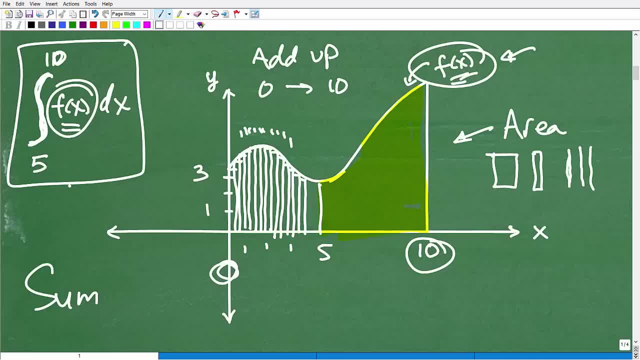 I would put a 5 right here and a 10 right there, and there you go Now how we actually calculate this mathematically. that's a little bit more involved- Not much more involved, but it's something that you can't handle. 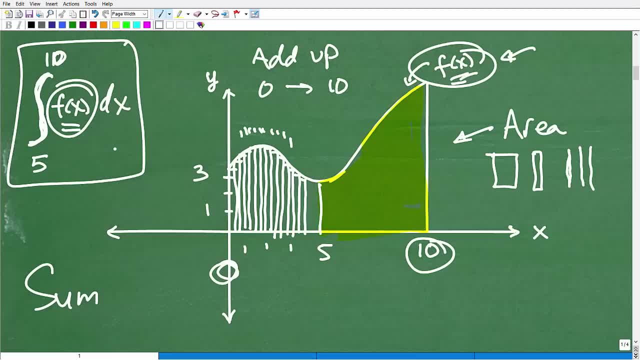 If I wanted to make this video a little bit longer, I could teach you how we calculate this. okay, But I just want you to understand the basic concept of calculus, This notation. it solves up finding the area of any crazy shape that you want, okay. 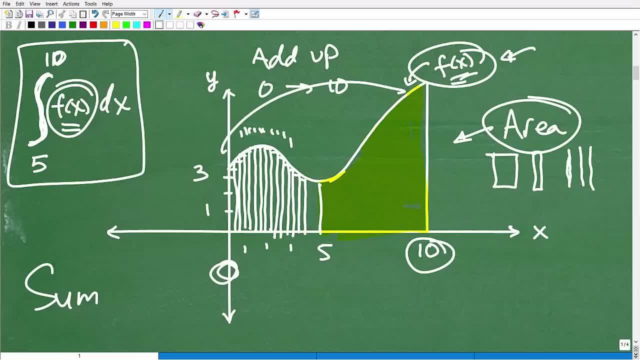 So if you change the function, you got a different kind of curve or something like that or whatever or something like this. It doesn't make a difference. We can find the area of anything we want- area and volume- using calculus, right? 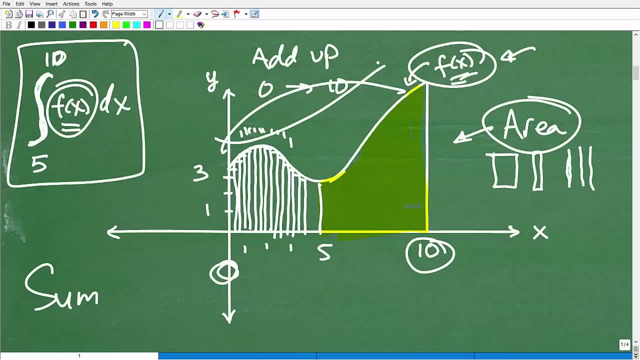 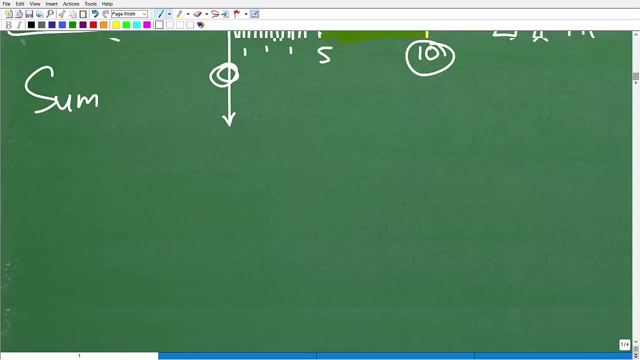 And we don't need a formula because obviously we don't have a direct formula for things like formulas for things like this. Okay, so that is the first Problem. calculus solves is like the area problem. Okay, let's get to the second problem. 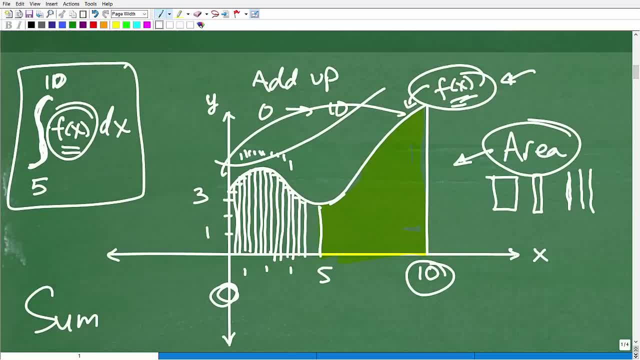 And, by the way, this is called integration using the integral. all right, that little fancy thing. Now you remember this right here, this little dx. all right, This is going to be the second kind of problem, That is, a derivative, okay. 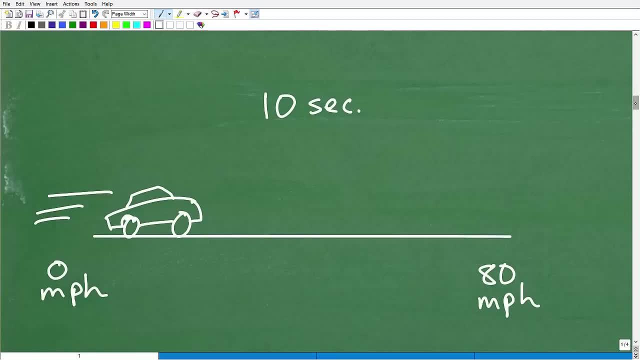 So the derivative is a little bit more. a little bit more, I want to say, difficult to explain, But hopefully, Hopefully, this example explains it All right. so the derivative dx: all right, over dy. you'll see that's symbology in calculus. 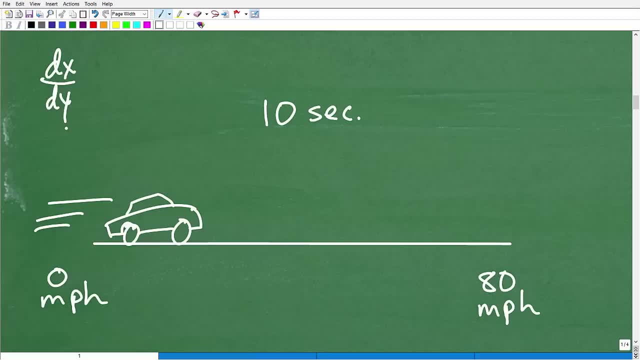 So there's two main things that calculus helps us solve. So the first one you can kind of think of is the area problem. We use that little integration symbol a to b I just showed you. And now the other problem is a little bit more sophisticated, right. 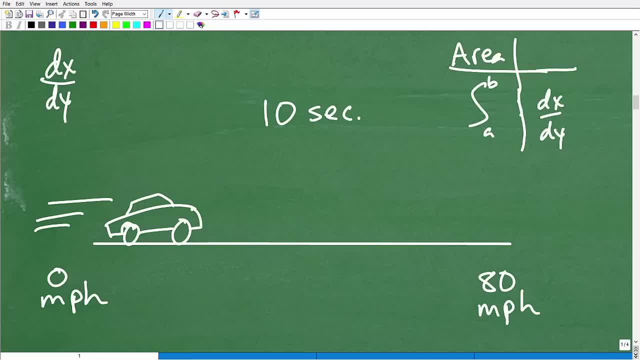 So this one is going to be dx, And you can kind of think of this as instantaneous velocity. Let me explain this to you. It's not that difficult to understand, but let me. I'm kind of rambling here, So let's get to this example, all right? 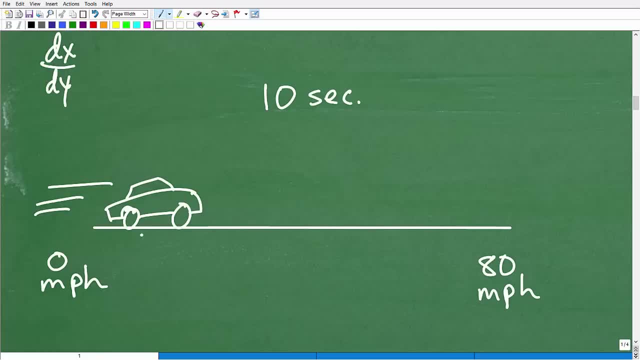 And then you'll understand it better. Okay, so here we have a car. Now the car is accelerating. okay, This car is taking off. Here's my little car. It's going faster, It's going right. So it starts at zero miles per hour and it's going to go increase its speed all the way up to 80 miles an hour. 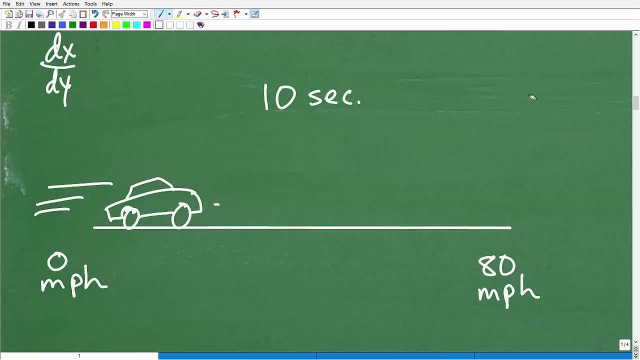 And let's say, it does this in 10 seconds. okay, So this is an accelerating car, accelerating car. So if I asked you, if I said, all right, from zero miles an hour, 80 miles an hour, and it does this in 10 seconds. 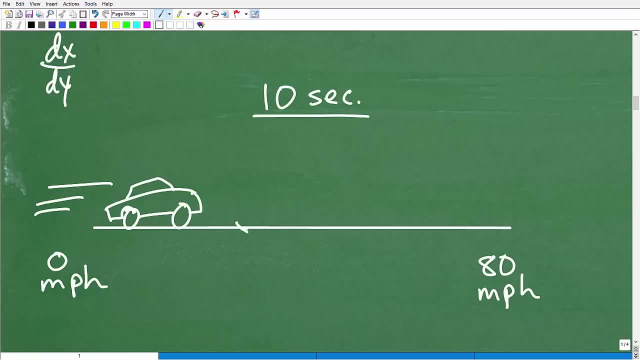 it said: how fast is this car going? at three seconds, Okay, At three seconds, into its little acceleration, how fast, What's? how fast is it going Okay? So you could say: well, it's at 10 seconds and you might use the formula rate times time equals distance. 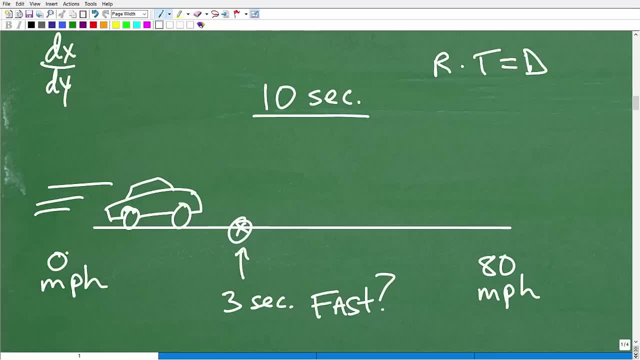 But precisely at three seconds. if it started at zero, it's obviously, you know, less than 80.. You might say: I don't know, maybe at three seconds it's going. you know, I don't know, Let's say 48.. 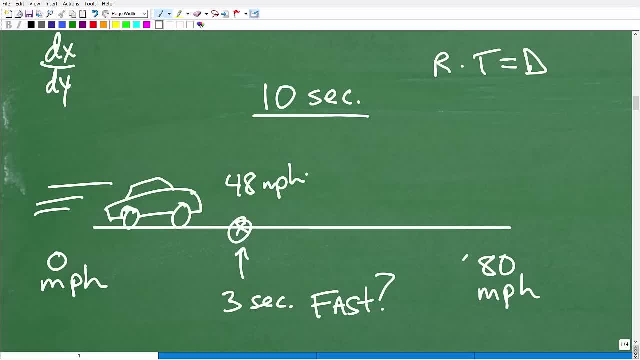 48 miles per hour. Well, how do we, how can we calculate that It's? if you think about it, the car is continuously increasing its speed. okay, You can't take the distance it's traveled, right and then divide it by its speed. okay, 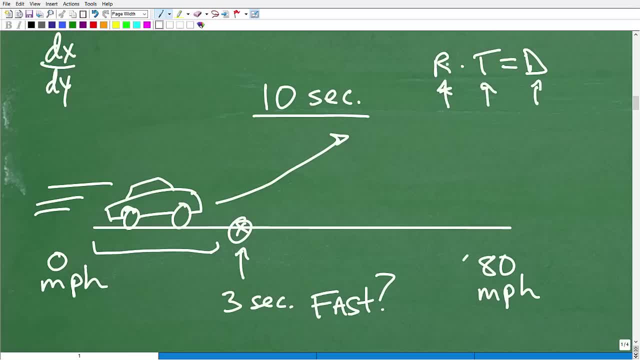 So rate times. time equals distance. This rate, this speed, okay, that's a fixed, that's a fixed velocity, all right, In other words, that's if this car was going 80 miles per hour down the highway, Let's say you know you're on the freeway and it's going 80, or the turnpike, whatever it may be located. 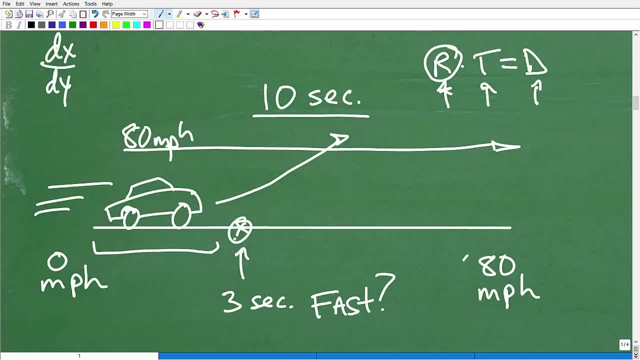 If it's going 80 miles per hour, you know all the way down the highway. then it's easy to. obviously it's going to be going 80 miles per hour the entire time, But it's easy to calculate. you know rate and distance problems because the velocity is the same. 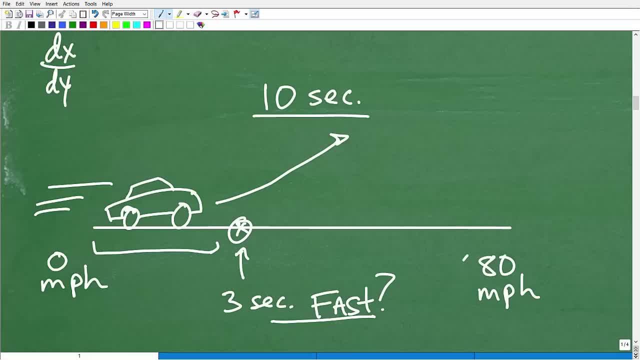 But when we're accelerating, how fast the car is going in this precise moment in time? that's a whole different ballgame. okay, We need calculus to be able to answer that question for us. So I might ask you: well, what about 5.12 seconds, okay, into this car's acceleration? how fast was it going? 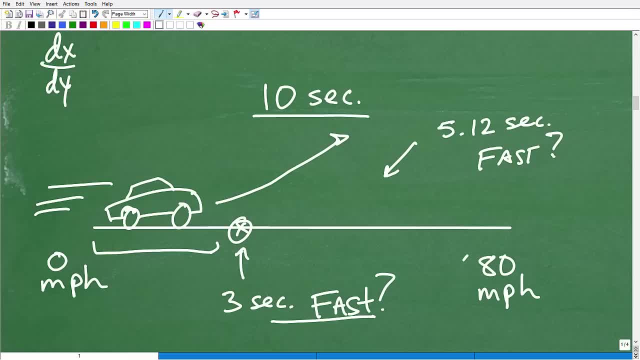 How fast was it going? okay, in that moment, precise moment in time. Well, in order, and this is an accelerating car, not a car that's going at a constant speed. So these type of problems to figure out the answer. 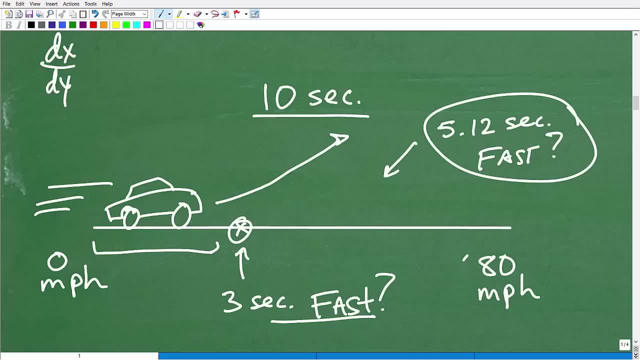 The answer to these instantaneous problems, like get a snapshot of what's going on at that precise moment, requires calculus. to be able to answer a question like that, We can't use average speed and time and distance, okay, That doesn't work in this kind of scenario. 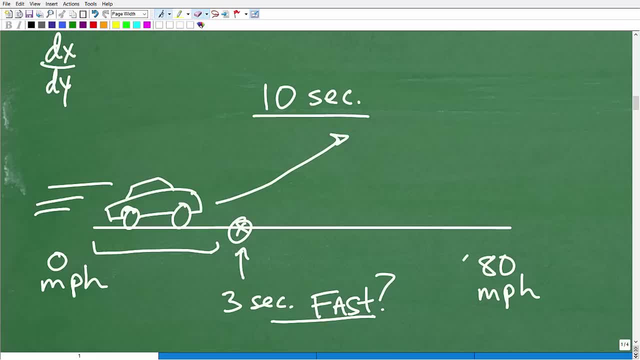 Let's see if I can give you another example to maybe make this a little bit better. So let's say I had like. well, let's say I'm doing an experiment, Say, this is the side of a building And I drop like a baseball or something, right, 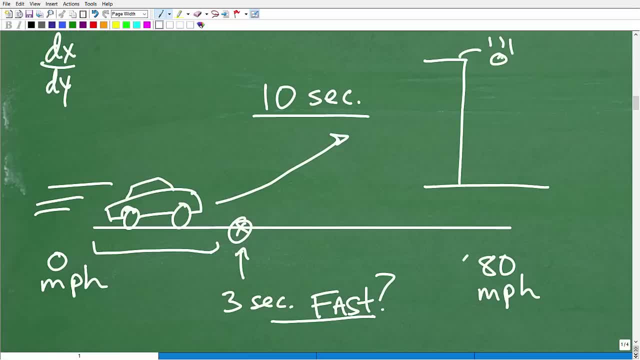 And I'm doing it safely. There's no one down here, And when I let go of the baseball, it's at zero miles per hour. okay, Now what's happening with the baseball? Well, it's picking up speed, picking up speed. 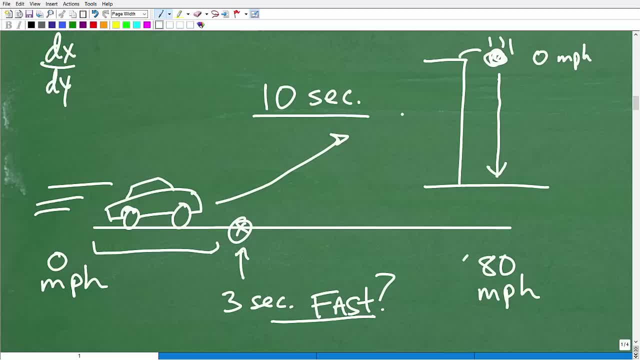 It's going faster, faster, faster, until it hits the ground right. Let's say this is 120 feet And, I don't know, maybe the baseball ends up going 120.. Let's see something different. Maybe it ends up going. 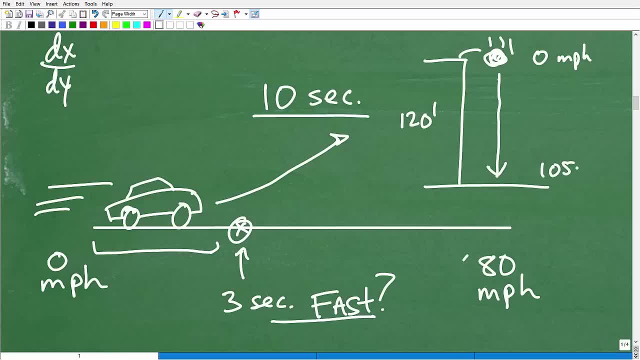 I don't know, 105 miles per hour by the time it hits the ground Now, and it took, oh, let's say, two seconds to do that. okay, So I'm just totally making up numbers here, But just to try to get the idea. 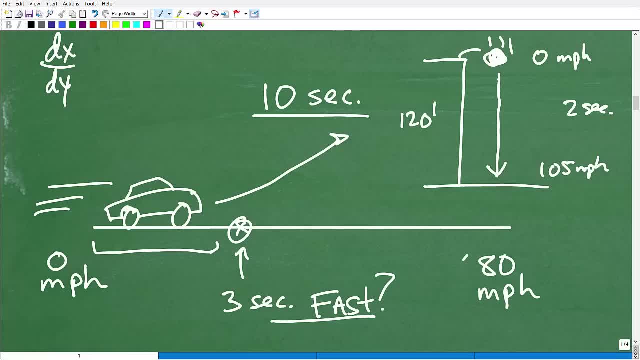 So if I let the baseball go- I didn't throw it, just let it go- it's starting to accelerate, right? I'm saying: well, how fast is a baseball going? at 0.78 seconds, right, How fast is it? 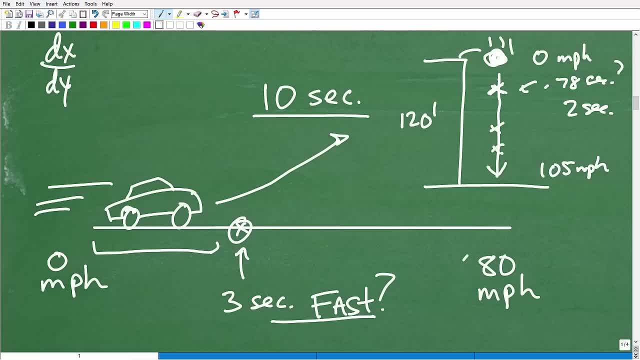 How fast is it going at this moment in time? this moment in time, this moment in time? okay, Well, again it's picking up speed, It's accelerating, But I want to know its instantaneous velocity at this, these little snapshots. 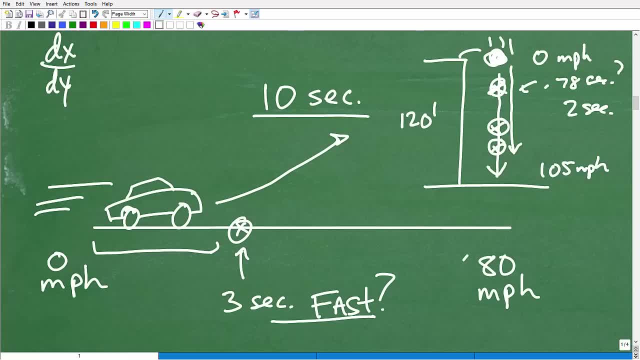 This requires calculus, okay, And this requires a concept of something called the derivative. okay, The derivative In calculus, a derivative, looks like that, All right. So calculus solves two big problems for us, right? It does so much more obviously. 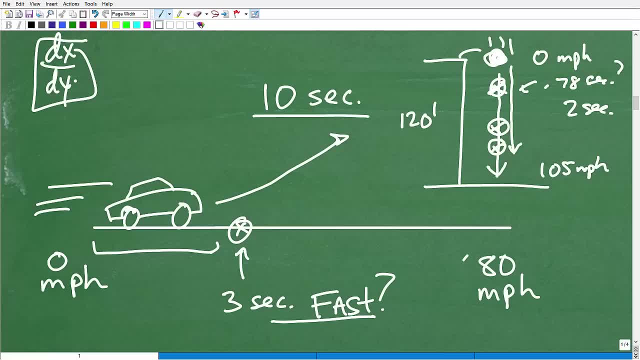 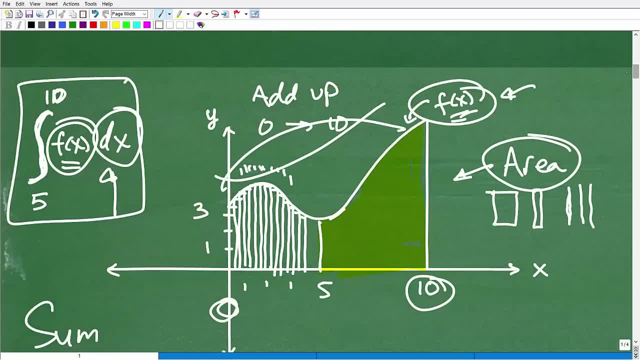 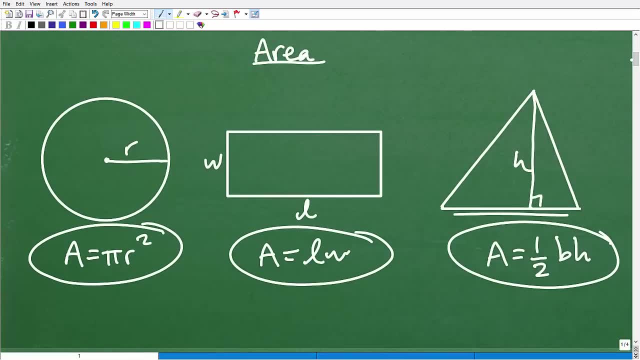 That's the first thing. The second thing is the area problem. okay, We can find the area of all kinds of crazy shapes, anything we want, And beyond the area we can find the area of volume, et cetera, And of course, calculus does even more than that. 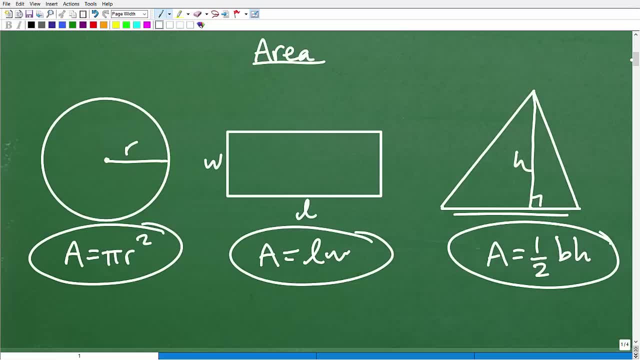 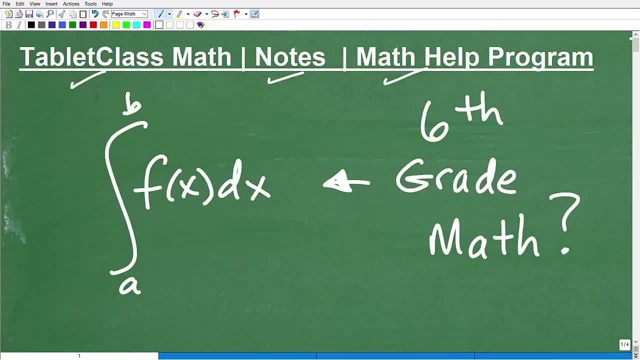 But if you didn't know anything about calculus, okay, and you understand this basic kind of math and you know the question about the car, then you got a pretty good feel for what the value of calculus, you know, does for us. 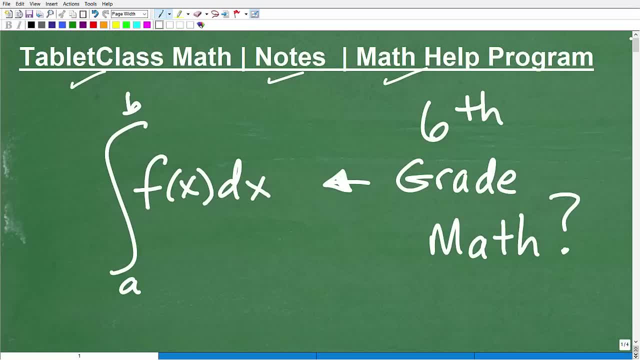 I hope I don't know where you're at in your math education, but you know I would certainly encourage anyone out there, everyone out there, to explore calculus. I know you're like I'm going to avoid it as much as I possibly can. 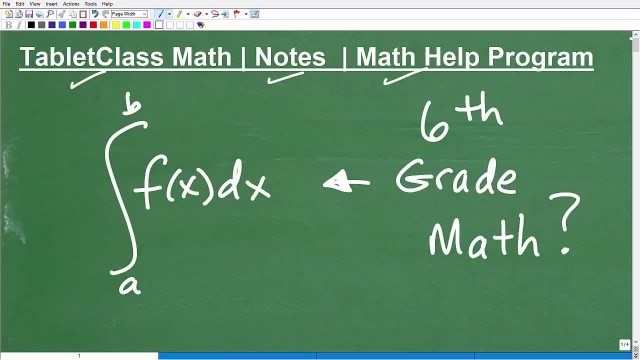 But if you could ever take this class, you know, pressure-free, you know- and just enjoy the concepts of it- yeah, there's a lot of challenging things to it. You know there's a lot of rules and other stuff. 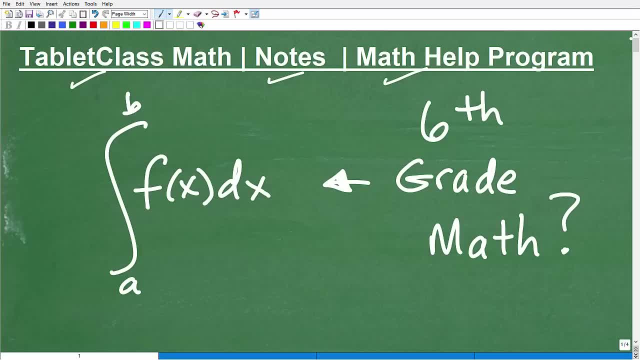 I'm not trying to minimize it, I'm not saying it's not a challenging math course, But the beauty of it is that it can solve such just awesome real-world problems for us. Okay, so that's it Again. if you need help with math, more instructional, full help, you know where to go. 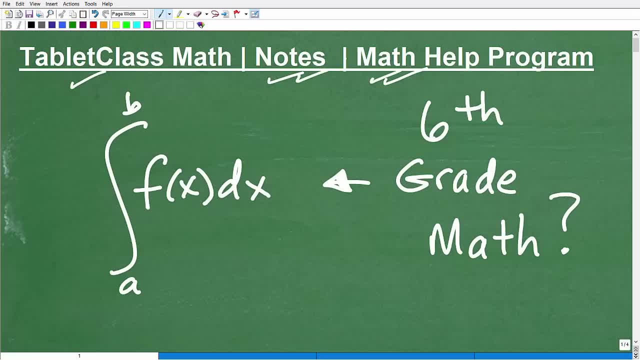 Just follow those links in the description of this video. Also, if you're new to my YouTube channel, I'm posting stuff all the time, so hopefully you'll consider subscribing. And, of course, if you like this video, please smash that like button.